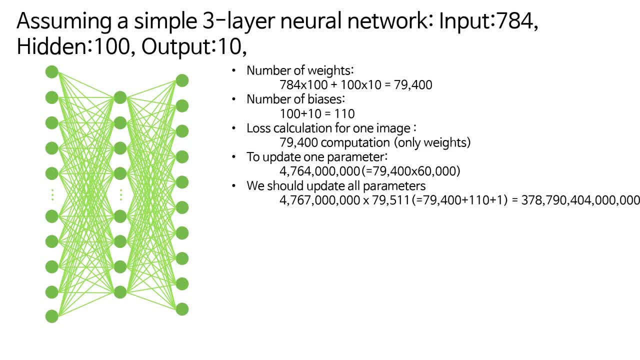 We need to compute for all parameters. This means 380 trillion operations just to update the gradient once. With a CPU processing speed of 850 million operations per second, based on i7-8750H, It would take 123 hours to change the weights of a three-layer neural network once, Finding the best. 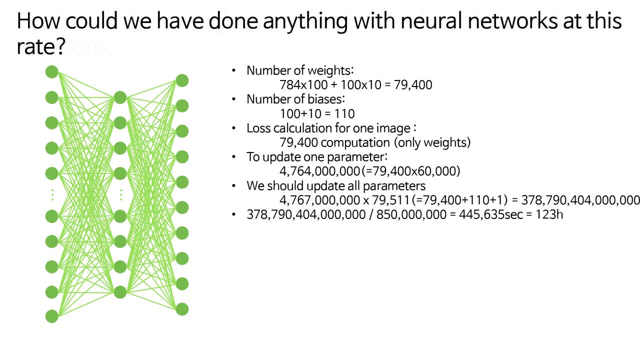 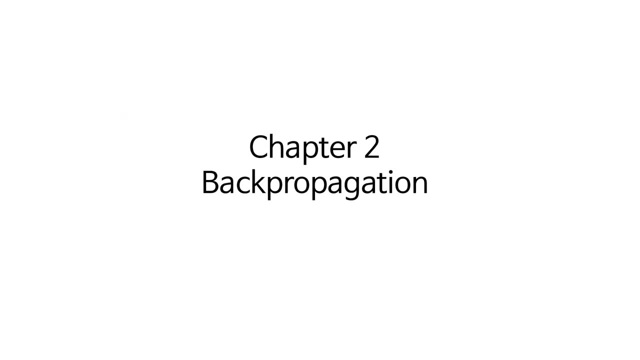 weights requires hundreds to thousands of iterations. How could we have done anything with neural networks at this rate? Without the backpropagation algorithm, the era of deep learning and AI would not have arrived. Chapter 2: Backpropagation. Now let's delve into the backpropagation algorithm. 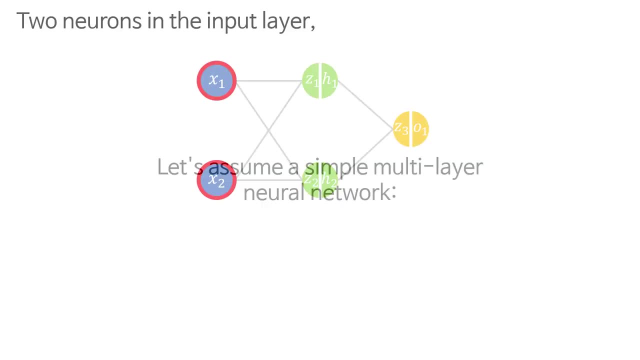 Let's assume a simple multi-layer neural network: 2 neurons in the input layer, 2 neurons in the hidden layer and 1 neur in the output formula- output layer- And there are six weights. We'll use the sigmoid function as the activation function. 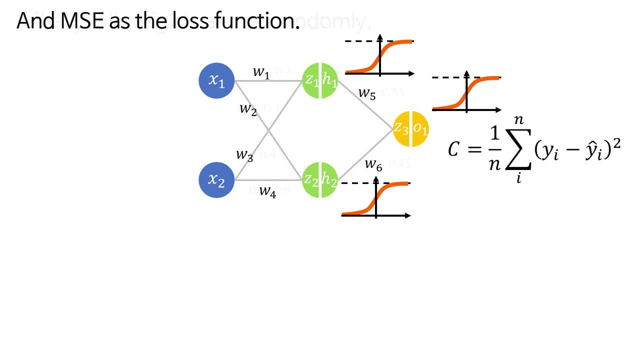 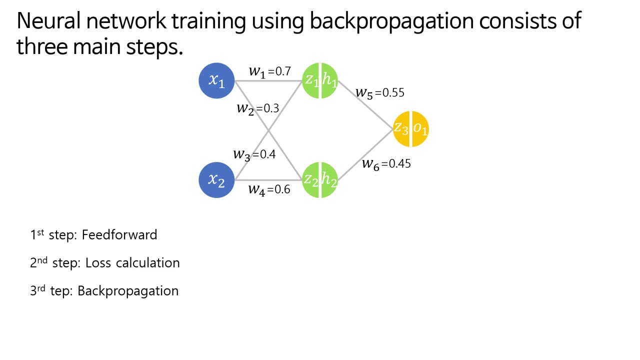 and mse as the loss function. Initially, all weights are set randomly and we'll assume a learning rate of 0.1.. With these settings in place, we're ready. Neural network training using backpropagation consists of three main steps. Repeating steps one to three helps us find the 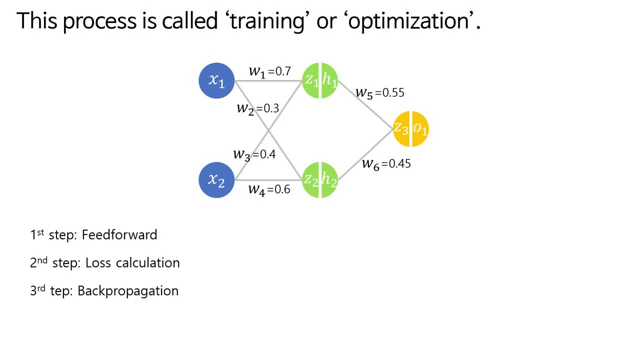 best parameters. This process is called training or optimization. Step one, the feedforward step, is straightforward. If, given certain input values, multiply them with the connection weights and sum them to get the hidden layer, node values, Then it's the turn of the hidden. 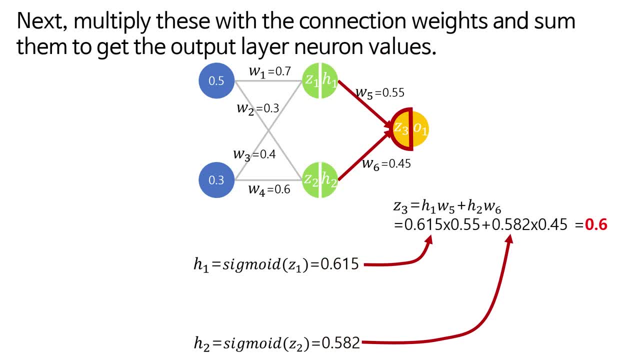 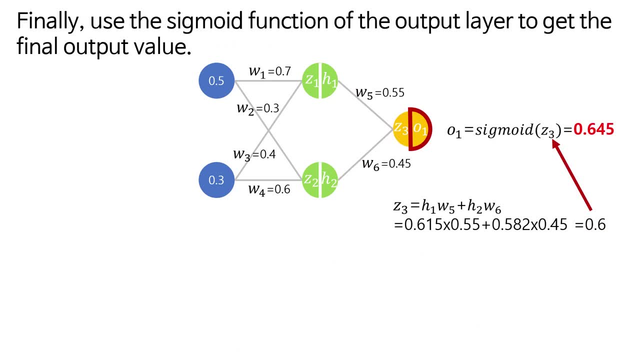 layer's activation function. Next, multiply these with the connection weights and sum them to get the output layer neuron values. Finally, use the sigmoid function of the output layer to get the final output value. This completes the feedforward step. The next step is calculating the loss. 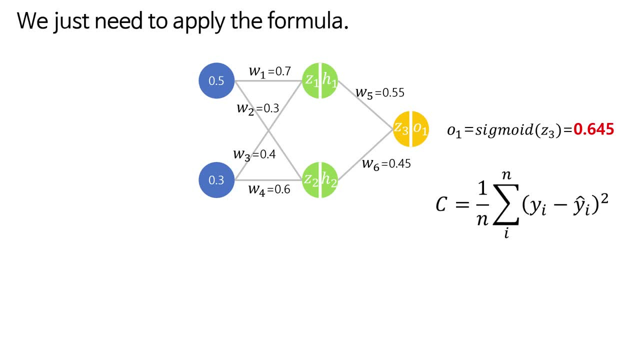 Since we're using mse, we just need to apply the formula. As there's only one output neuron, the formula becomes mse. If we assume an output value of 0.645 and a real value of 1, the error c is 0.126.. 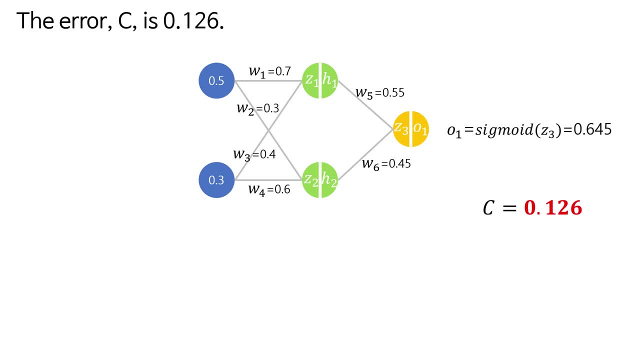 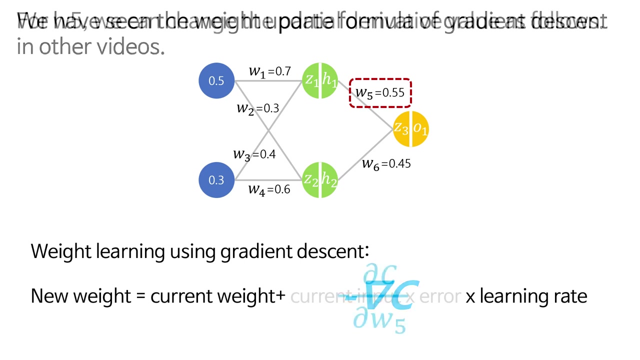 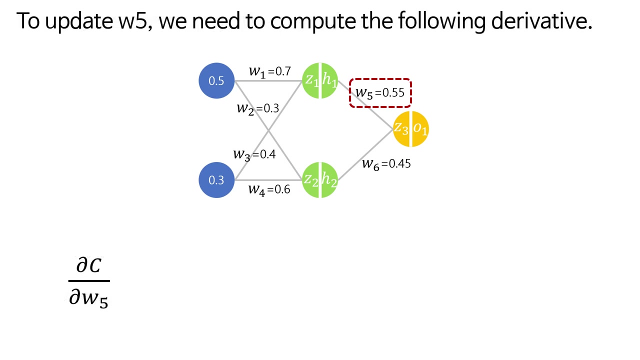 Now the last step: backpropagation. Let's start by updating the weight w5.. We have seen the weight update formula of gradient descent in other videos. For w5, we can change the partial derivative value as follows: To update w5, we need to compute the following derivative: However, since we can't, 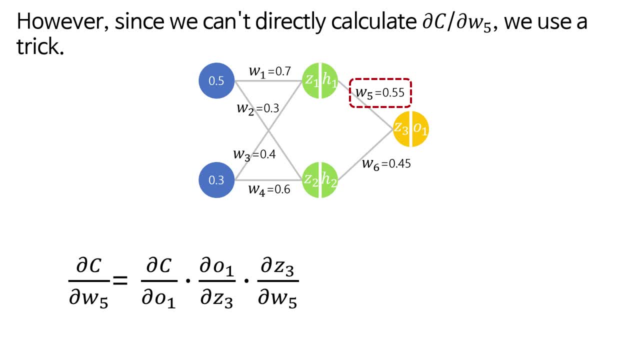 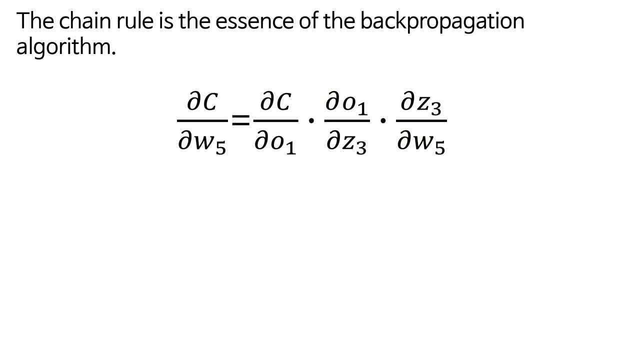 directly calculate del c, del w5,, we use a trick. This is known as the chain rule. The chain rule is the essence of the backpropagation algorithm. When we want to differentiate a function with respect to two variables but don't know their relationship. 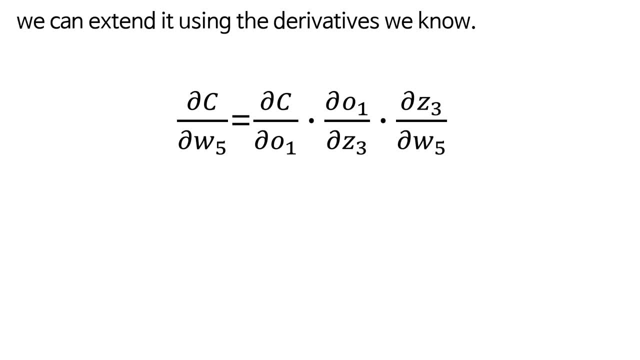 we can extend it using the derivatives we know. By addressing parts of the problem, we can potentially solve the whole problem. Eventually, only the relationship we want to understand remains. The mathematical proof of the chain rule might be challenging, but understanding the concept isn't so difficult. Consider this example. 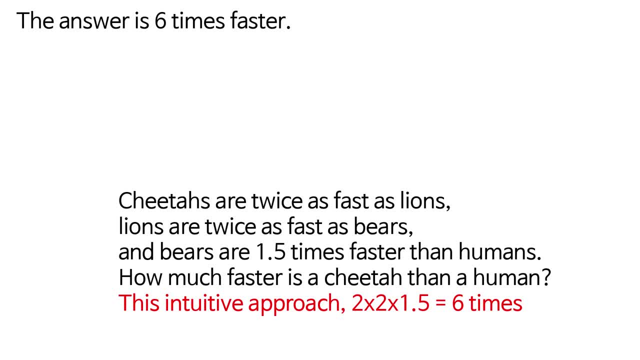 Cheetahs are twice as fast as lions, lions are twice as fast as bears and bears are 1.5 times faster than humans. This means that they are twice as fast as humans. This means that they are twice as fast as humans. How much faster is a cheetah than a human? The answer is six times faster. 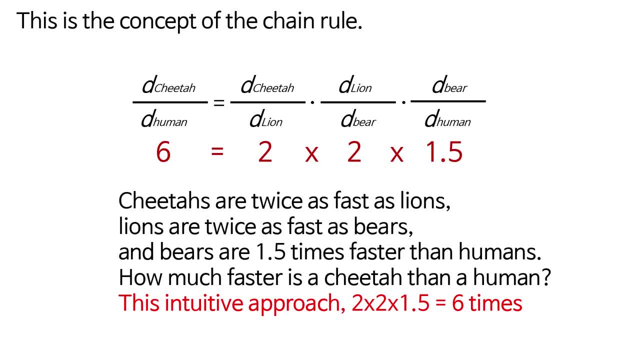 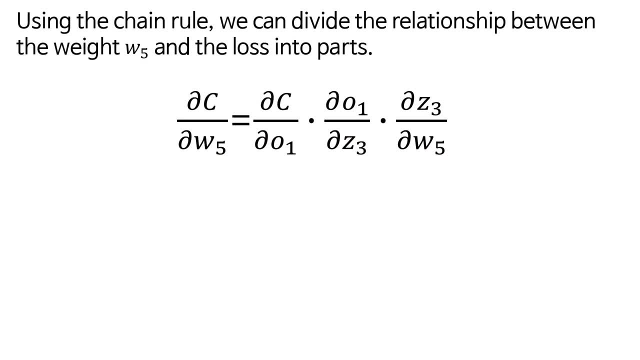 This intuitive approach- two times two times 1.5 is equal to six times- is the concept of the chain rule. Using the chain rule, we can divide the relationship between the weight w5 and the loss into parts. This is the essence of the backpropagation algorithm, So let's compute each part. 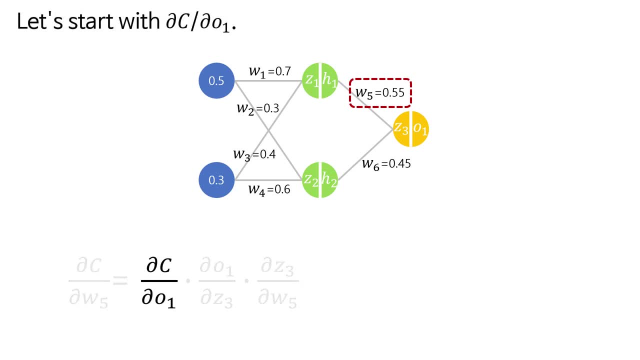 Let's start with del c del o1.. Our loss function can be represented as follows: Differentiating the formula with respect to o1 gives With an o1 value of 0.645.. When we plug in the actual values and compute, Del c del o1 is minus 0.71.. Next we'll compute. 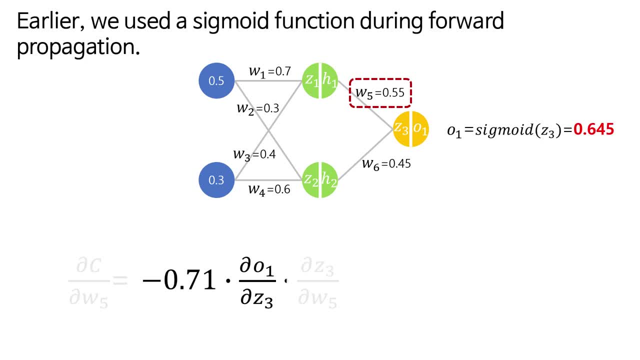 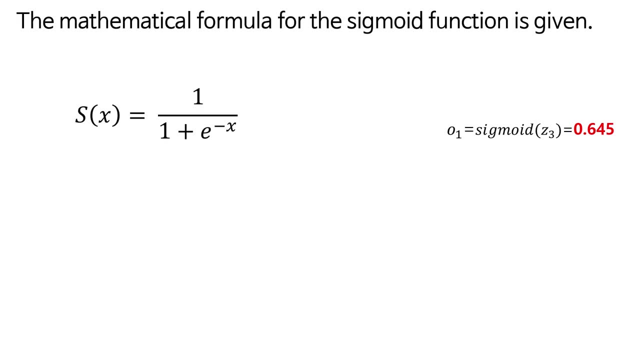 del o1, del z3.. Del c del o1 is minus 0.71.. Next we'll compute del o1, del z3.. Earlier we used a sigmoid function during forward propagation. The mathematical formula for the sigmoid function is given: 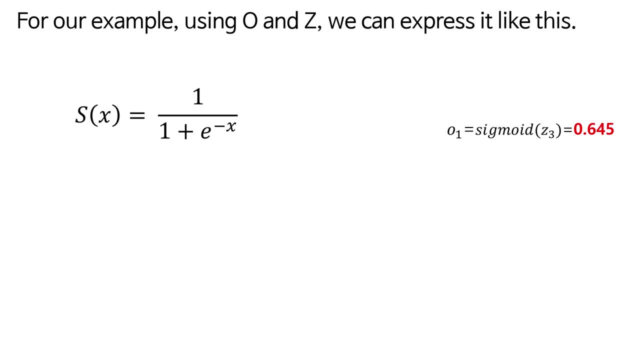 For our example, using o and z, we can express it like this: By changing the variables, we can rewrite it. Let's find the derivative of the sigmoid function for z. I'll skip the complex differentiation process. The derivative is simple and looks like this: 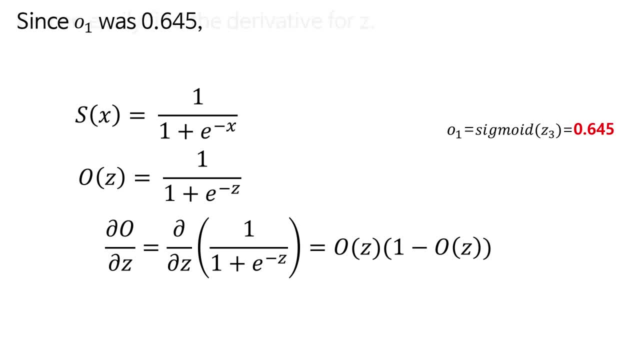 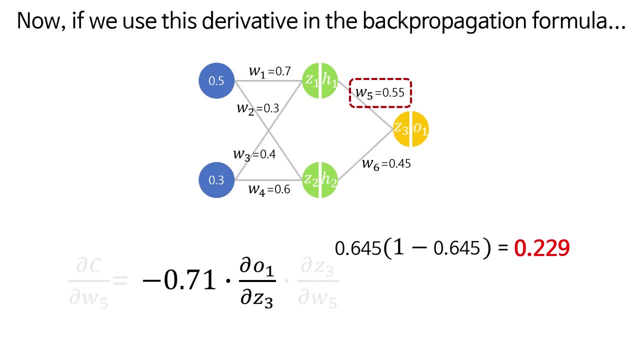 Since o1 was 0.645,, we can easily find the derivative for z. Now, if we use this derivative in the backpropagation formula, We can find the second term. Next, let's find the third term del z3, del w5.. Finding the third term del z3, del w5, is straightforward, Since z3 was a sum of. 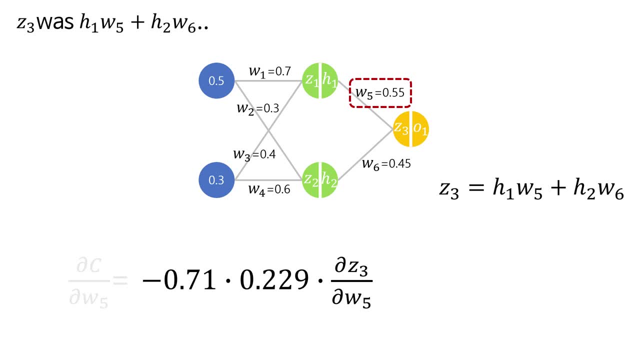 terms with h1 times w5 and h2 times w6.. Differentiating z3 with respect to w5 gives h1.. From our forward propagation, h1 was 0.615.. Using this value, we can compute del c del w5.. 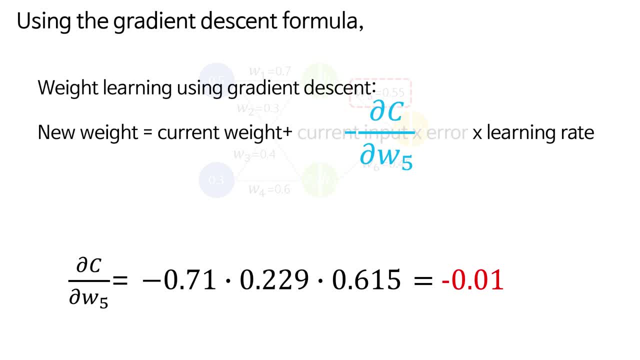 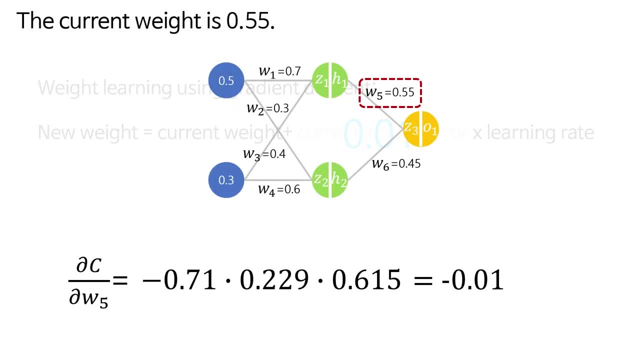 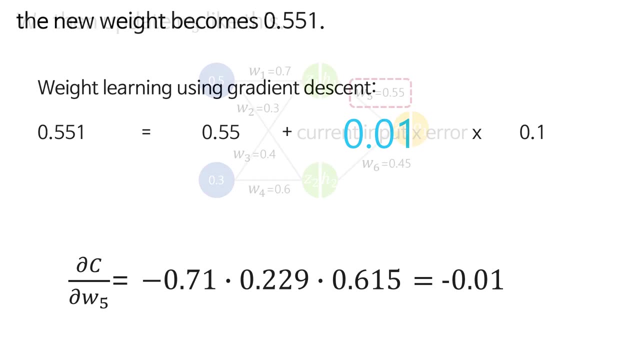 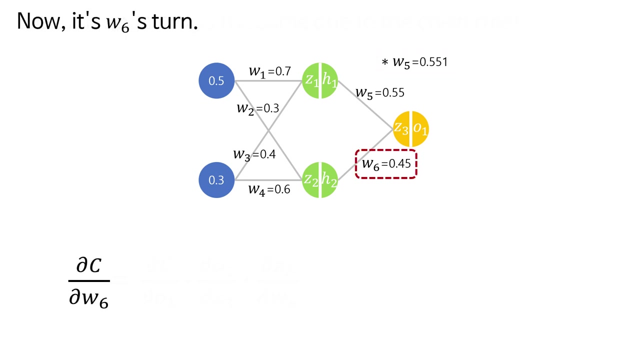 Using the gradient descent formula, we update the weights. We can input the gradient like this: The current weight is 0.55.. With a learning rate of 0.1, the new weight becomes 0.551.. We then update w5 like this: Now it's w6's turn. The process for w6 is the same, due to the chain. 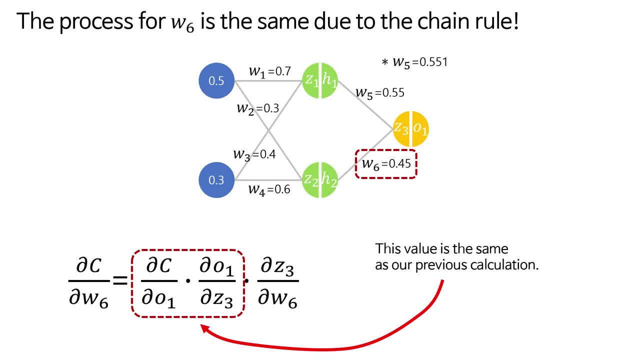 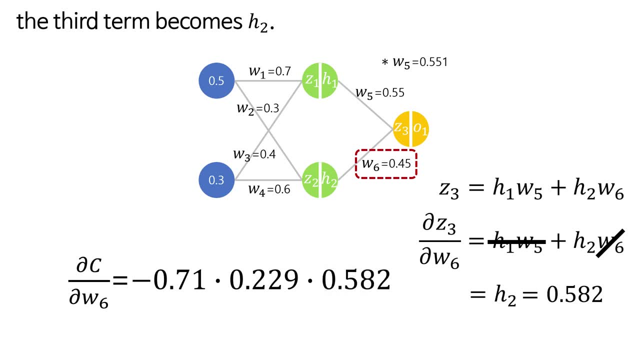 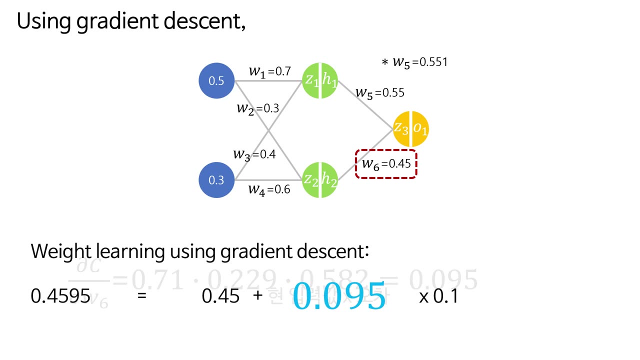 rule, This value is the same as our previous calculation. Using these values, the third term becomes h2.. Thus, del c del w6 is minus 0.095.. Using gradient descent, w6 updates to 0.4595. 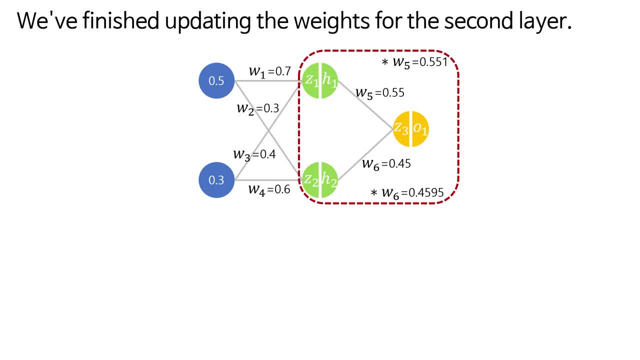 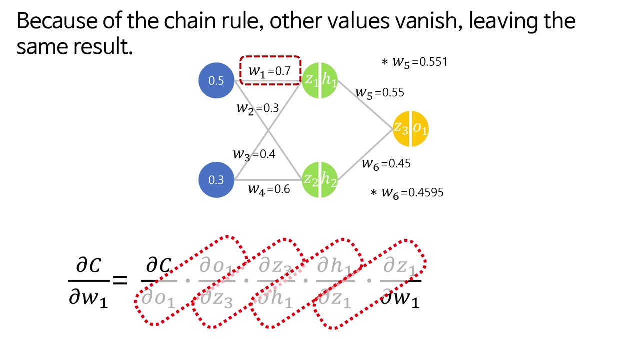 We've finished updating the weights for the second layer. Let's move to the first layer. The process for w1 is the same due to the chain rule. We can express w1 like this: Because of the chain rule, other values vanish, leaving the same result. This value is the same as our previous calculation. 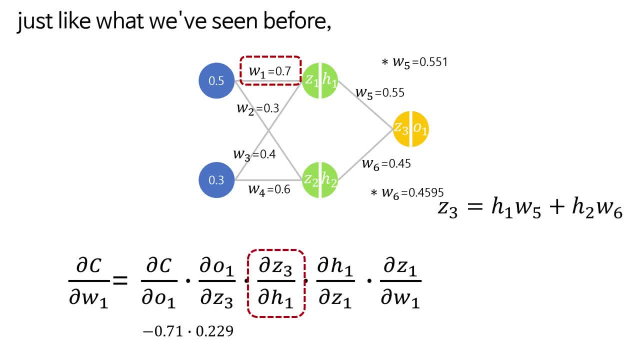 And for the part del Z3, del H1.. Just like what we've seen before, We can reuse the already calculated value of W5.. The value of del H1, del Z1 is the derivative of the sigmoid function. We can use the H1 value we already calculated during the forward propagation. 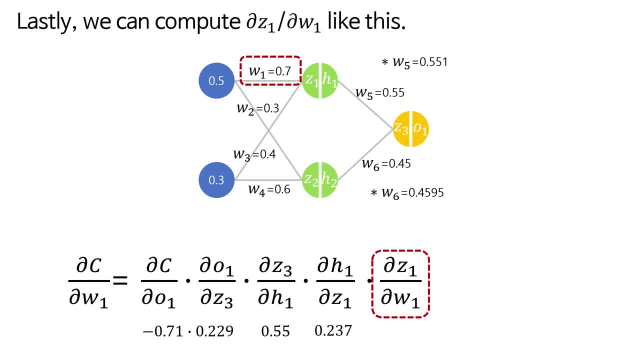 to compute it. Lastly, we can compute del Z1, del W1 like this: During forward propagation we computed Z1 in this way: If we differentiate it, the final term becomes the input value X1.. Using this, we find del C del W1 to be minus 0.01.. 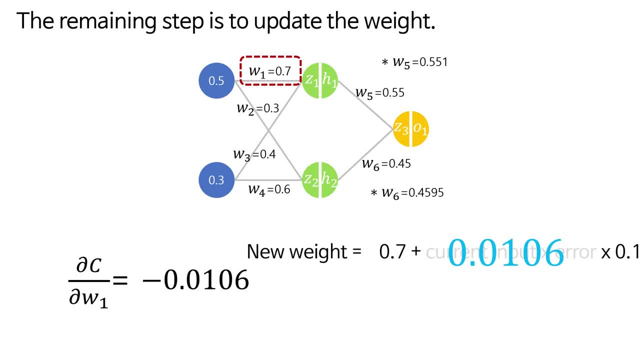 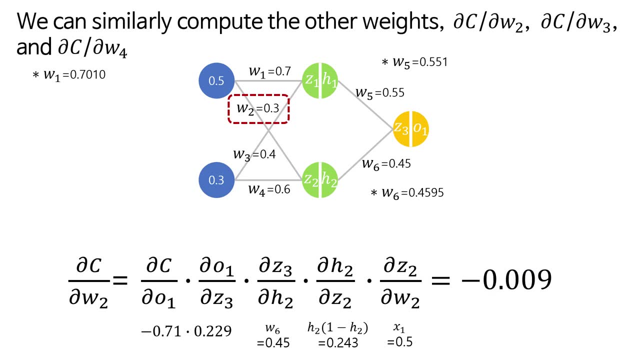 The remaining step is to update the weight. W1 becomes 0.7010.. We can similarly compute the other weights del C del W2, del C del W3, and del C del W4.. We can update each of these weights accordingly. 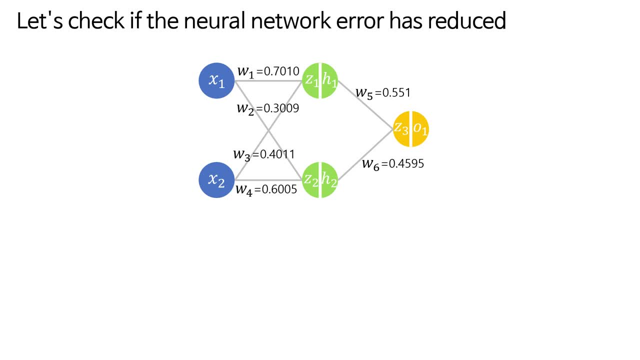 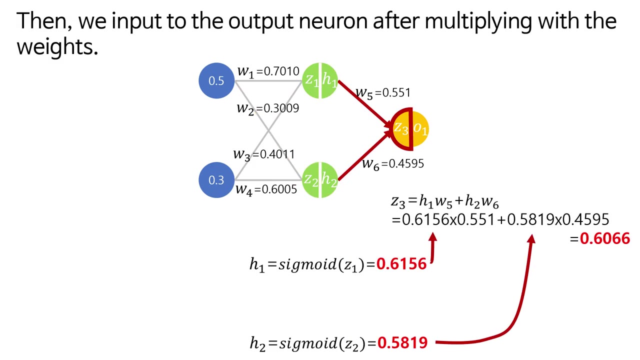 Let's check if the neural network error has reduced using the backpropagation algorithm. Let's input the same values again. We add the weights and input them to the hidden layer node. Next is the activation function for the hidden layer. Then we input to the output neuron after multiplying with the weights. 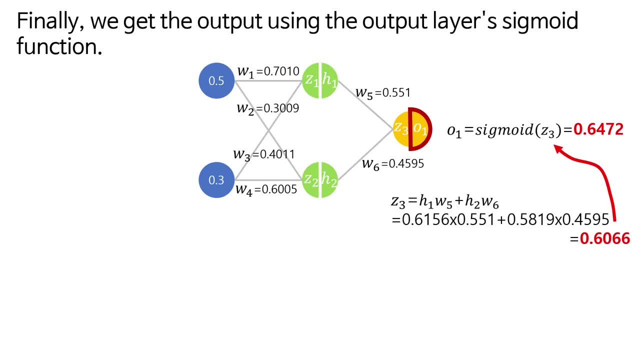 Finally, we get the output using the output layer's sigmoid function. Then the forward propagation is complete. Considering the last step, the loss function, Let's contexts the process of output expression with the sequence function. Let's add the values to the output neuron after multiplying with the weights. 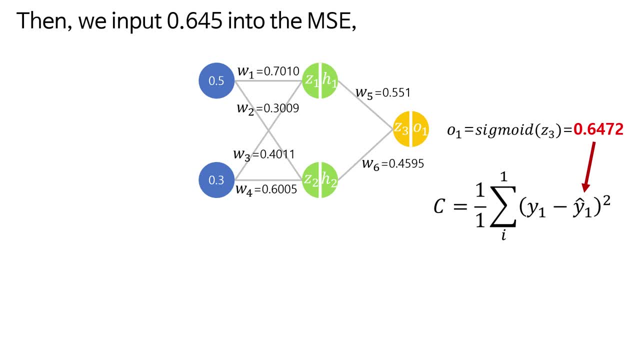 Finally, we get the output using the output layer sigmoid function. Then we put all the values in a new С function. then we input 0.645 into the mse and assume the real value is 1.. we get an error c of 0.1245. 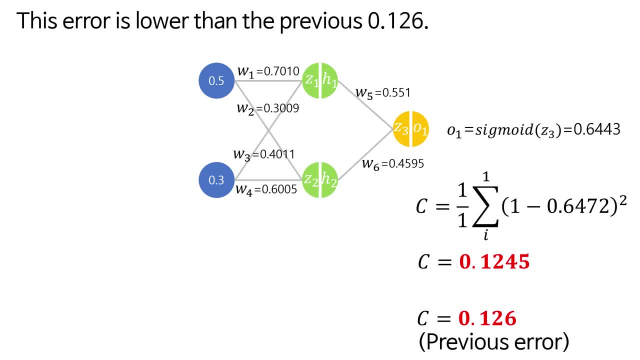 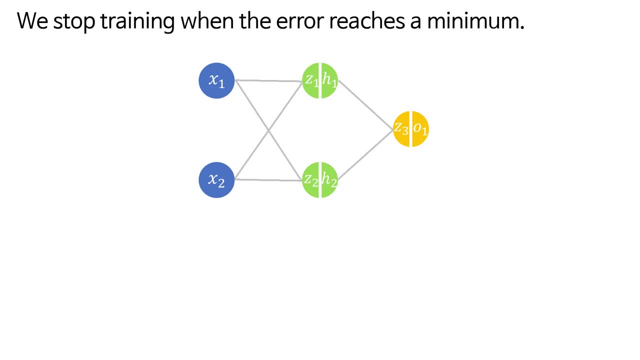 this error is lower than the previous 0.126, we repeat the forward propagation, loss calculation and back propagation. we stop training when the error reaches a minimum. that concludes our tutorial on the back propagation algorithm. the key to back propagation is the chain rule and partial differentiation.